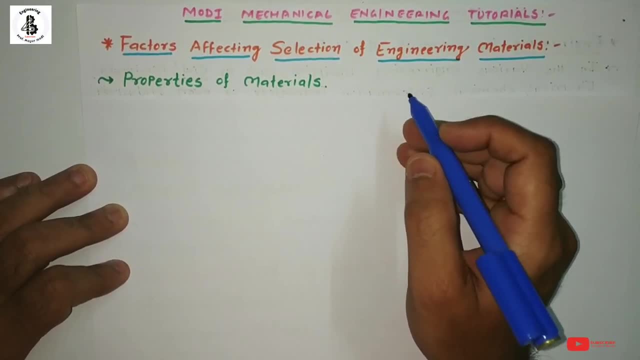 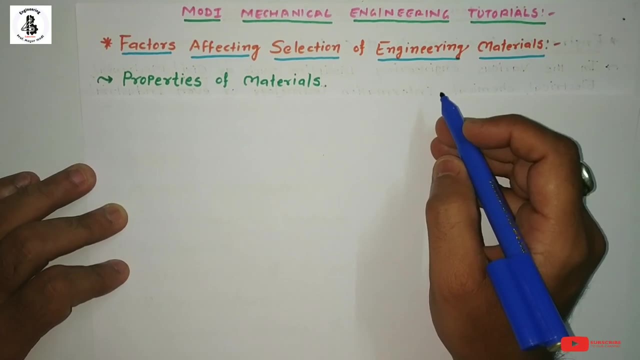 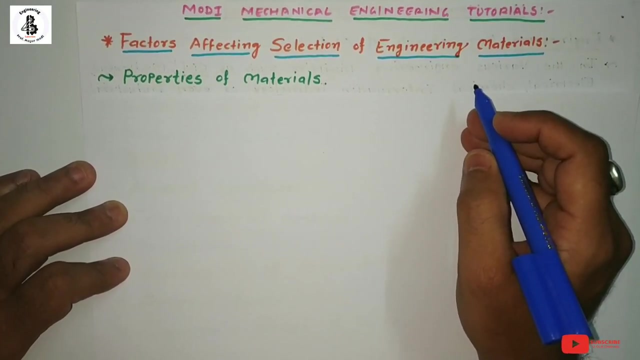 So that materials it will be sustaining all kind of under the loading conditions, or you can say different loading conditions. So basically the importance property of the materials that will be like as a mechanical properties. Then considering as a strength, hardness, that all considering as a mechanical property. 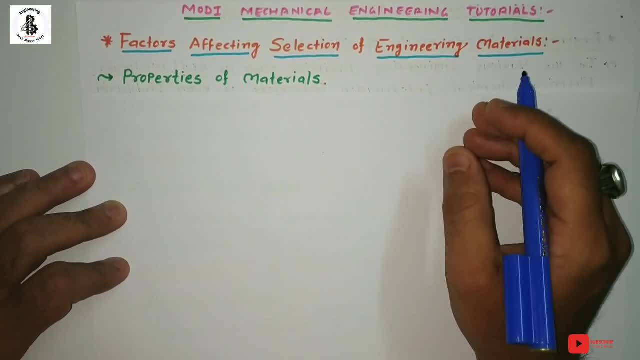 If you want to want on to the electrical properties like conductivity, resistivity, If it will be the thermal properties like heat capacity, heat or you can say thermal conductivity. Then if you want to want the electrical properties like conductivity, resistivity work on to the magnetic properties like hysteresis, then magnetic fields or magnetic flux that will be. 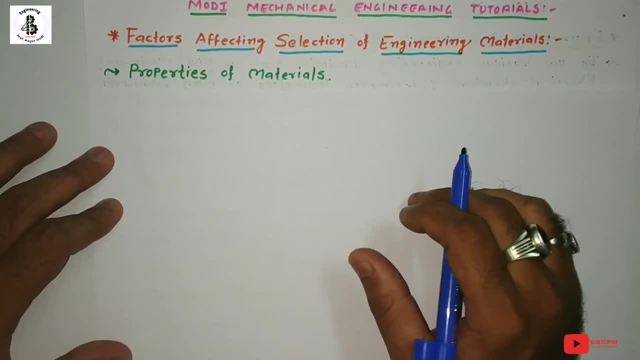 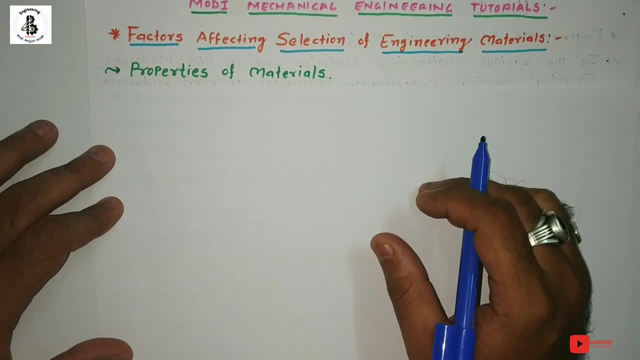 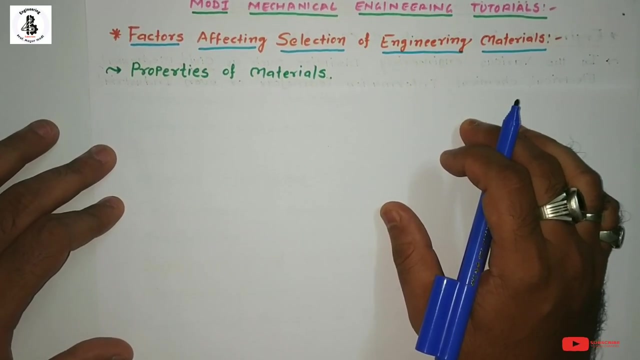 considering for the magnetic properties, chemical properties like electron affinity, electron negativity and acidity etc. for the optical properties like reflection, diffractions, absorptivity etc. so basically, which kind of factors- or you can say properties- is being required for the engineering materials? so in the field of the engineering there are different kind. 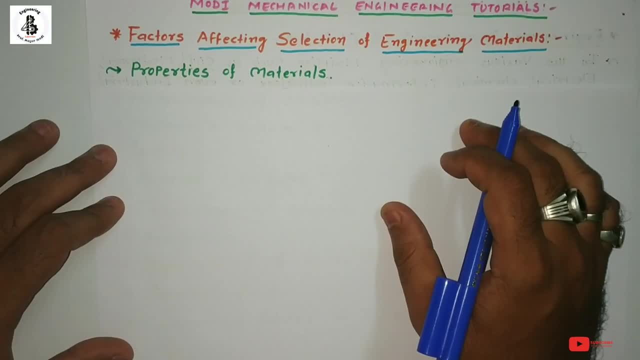 of products and different kind of products. it will be having a different kind of properties. so, as per the requirement of that particular products we need, or that will be the necessity of, the different kind of properties is being present into the materials. so the first one that will be the 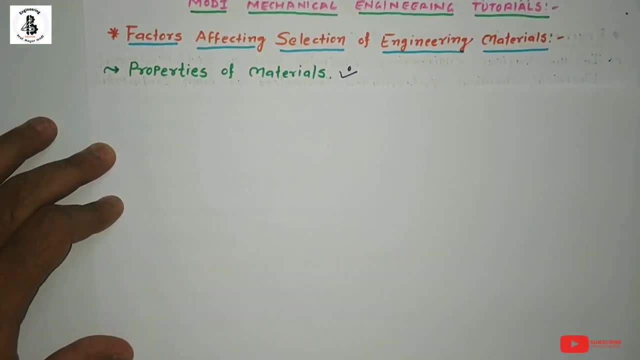 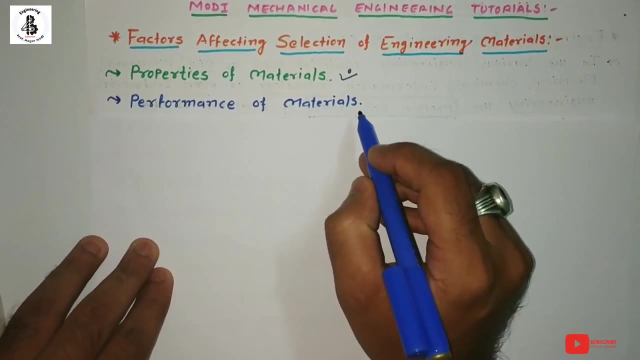 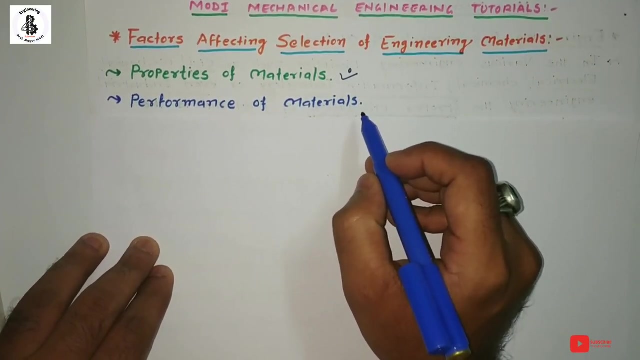 you properties of the material. that will be the important part for selection of engineering materials. then second one, the performance of materials. so basically, the components made of of your selected material must be having a capability of performing the functions assigned to without the failure, or you can say, without failure it will be having a good performance. 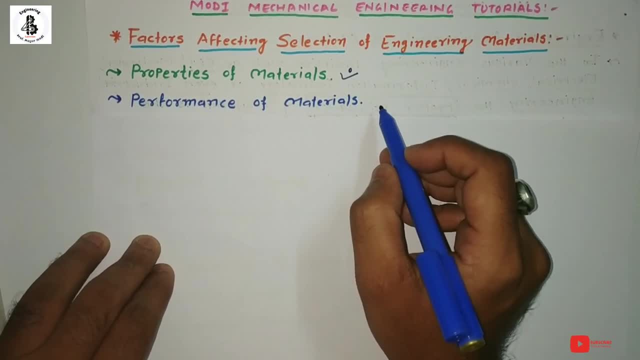 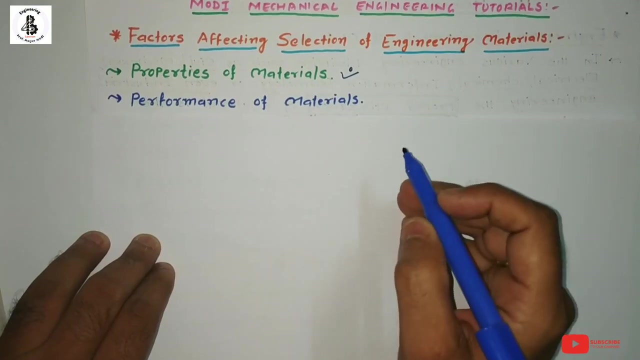 or you can say satisfactorily, performance, Like a box room, so which one has a hard and sharp angle. so, whether it is a good or a 30 degree angle, may let me show it? so right, yes, the article, that was quite the example I'll give myself. so let's take, for example, a brief example that has been given to us, when we used to generate a popsicle, Well, let's say the right cycle during the cycle, then all the revealed components or components. so basically the performance is a qualitative kind of functional types. so it is be related precisely what is specified, the values of the فahhac coverage, such as mechanical, thermal, physical, etc. So I will give a little examples, a part to be stewed. 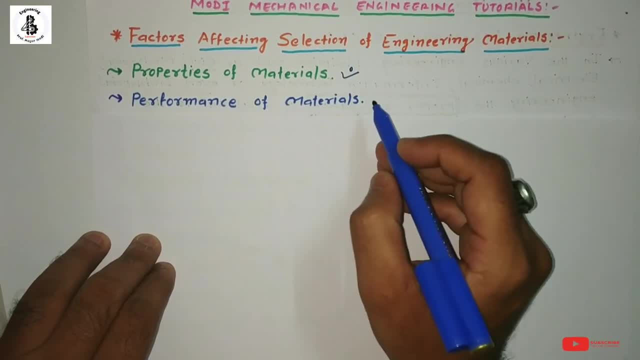 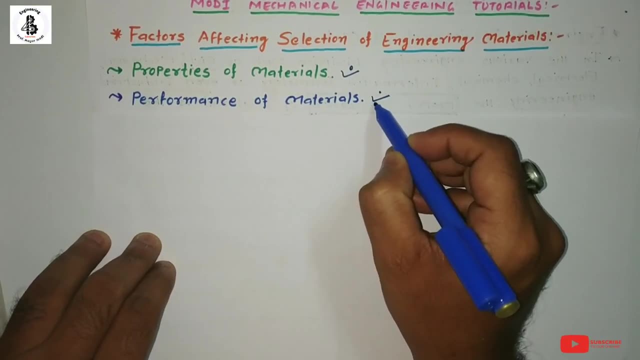 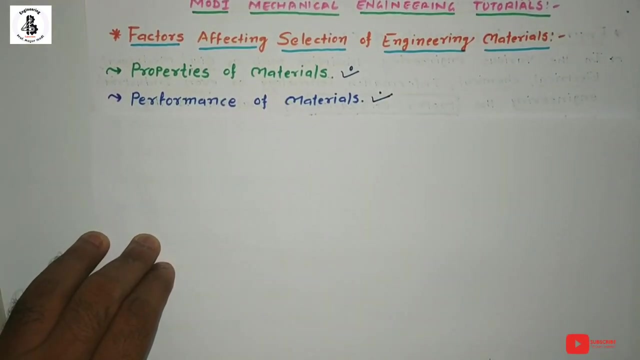 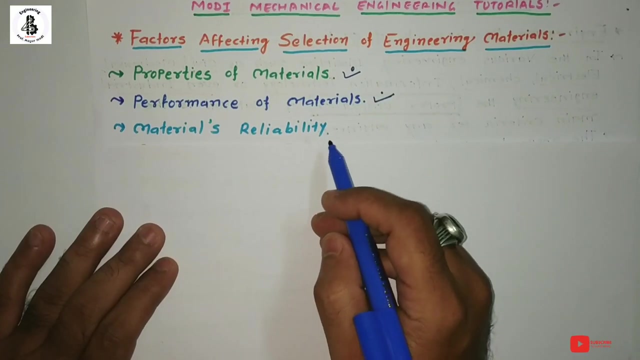 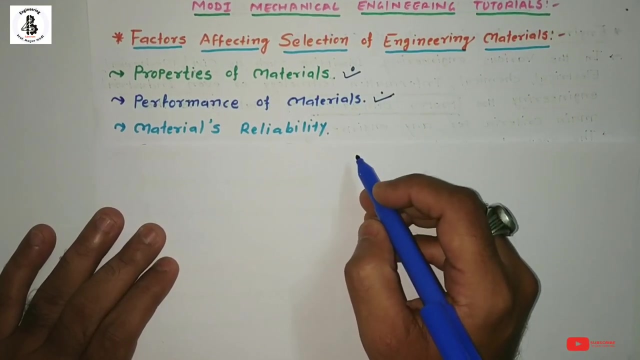 so the most important part for selection of the engineering materials, that will be the performance. so each and every components, process or you can say any kind of methodology, it will be check its performance level. then next materials reliability. so reliability is the degree of probability that a product and its material will remain stable enough to function in service for. 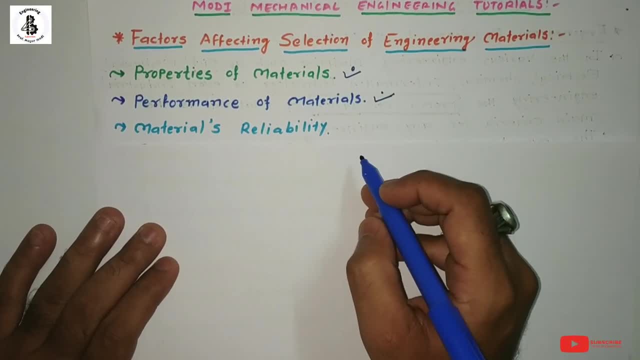 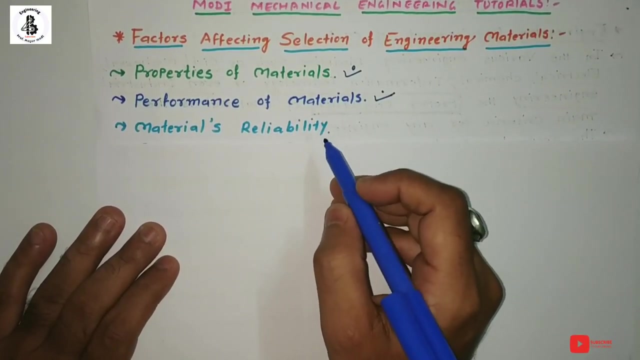 the intended life of the product without failure. so a material in a given applications must be reliable for its functionally so it never changes the performance of the products with it will be having a highly reliable. so it will be some drastically change into the loading capability. so it will be some drastically change into the loading capability so it will be some 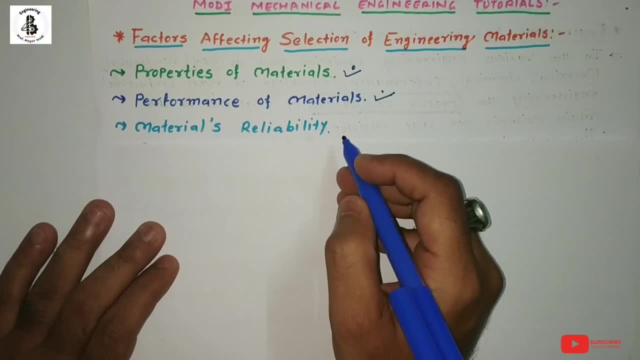 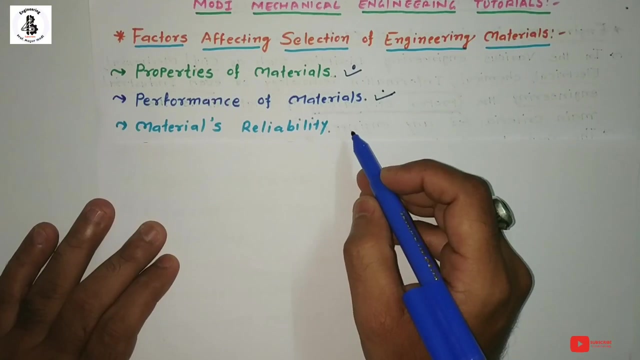 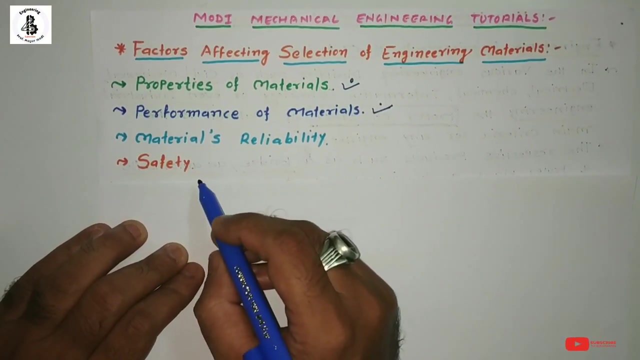 conditions, so that material must be reliable to give its best performance during the working conditions. so that will be the basic requirements of the materials. reliability. so by that reliability it will be reduced the accidents during the operation of the any kind of product. safety. so safety implies here for the human beings as well as place where the material is being used. 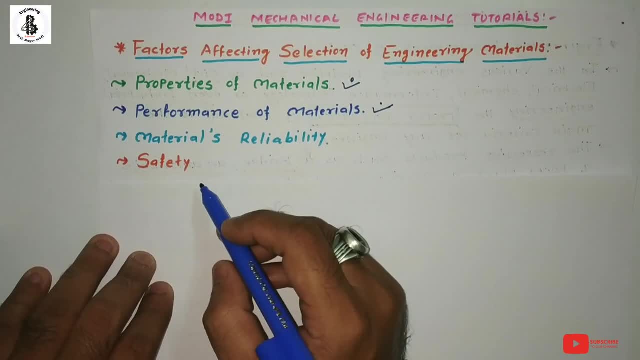 safety. so safety implies here for the human beings as well as place where the material is being used as a part of a product. so a material must be perform its functions safely. otherwise the failure of the product made out of these material may result in a great loss of the lives in the form of the human. 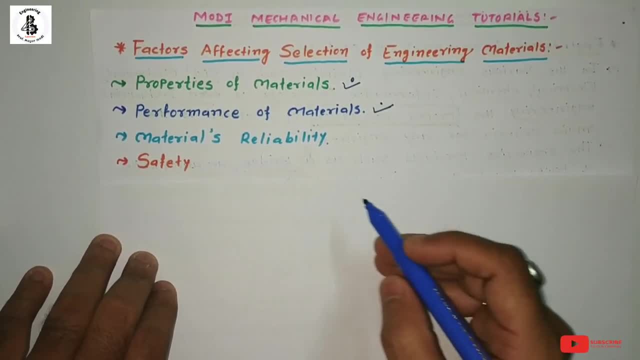 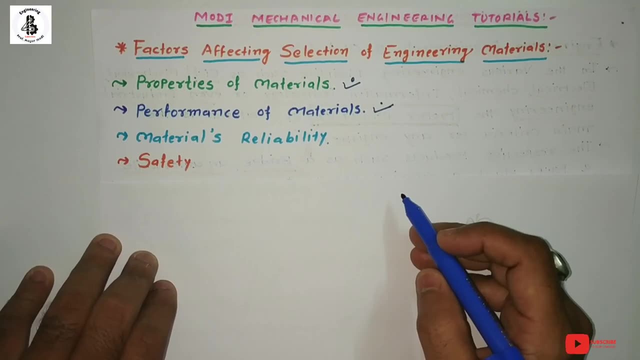 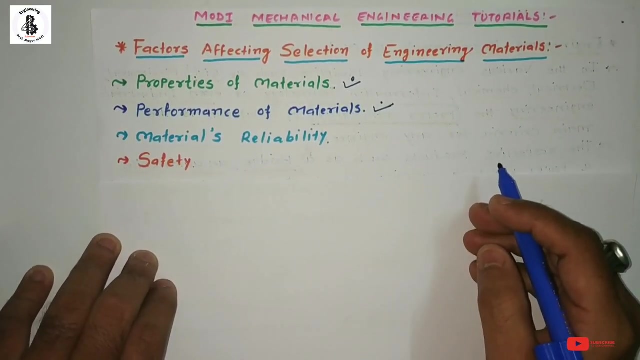 beings, as well as properties in the form of equipments, building, etc. so that will be having highly safety. it will be required for the products of the materials and as well as the for the human beings. so by the application of the safety you should reducing your accident during the processing or you can say use of that particular engineering products, physical. 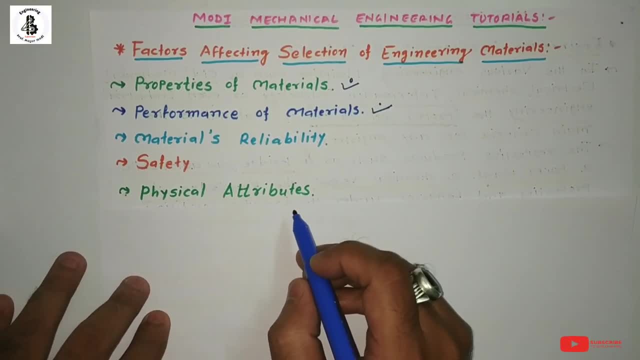 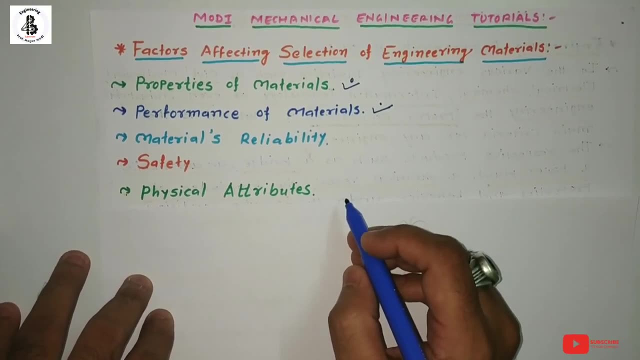 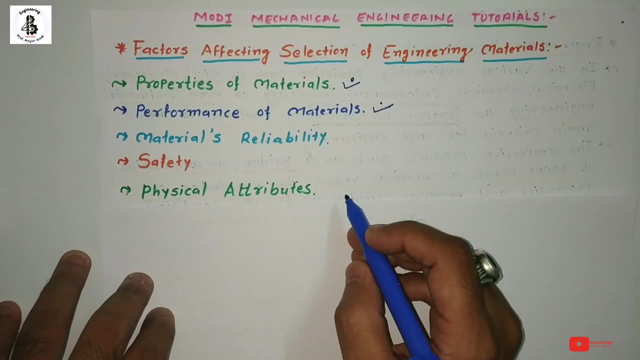 attributes, so the factors such as dimensions, mass, volume, color, appearance, etc. which will be affect the selection of the materials in many ways. so nowadays most of the people- or you can say customers- that will be more focusing on to the physical attributes. so they affect the service as well as the safety requirements of the product into the service conditions. so that will be the 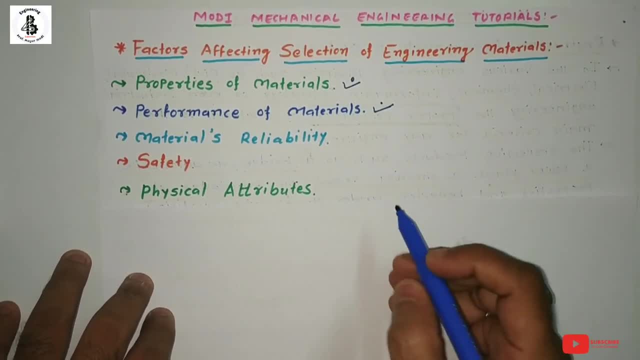 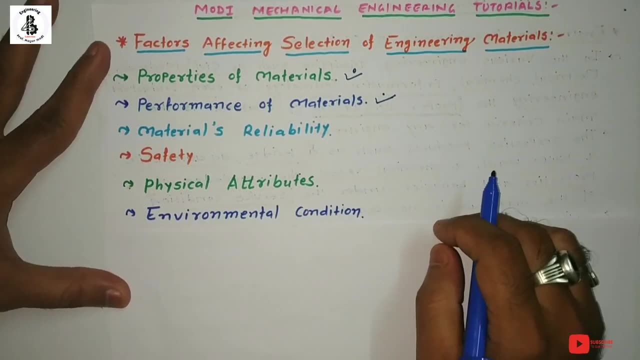 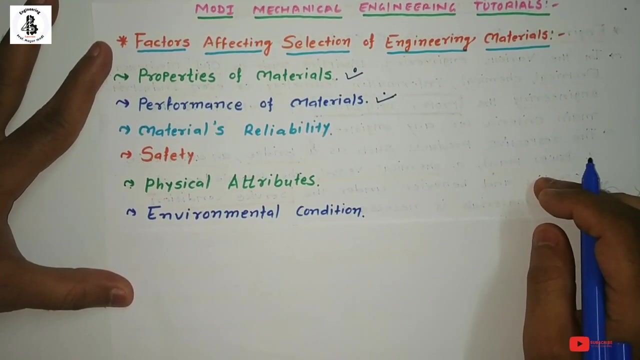 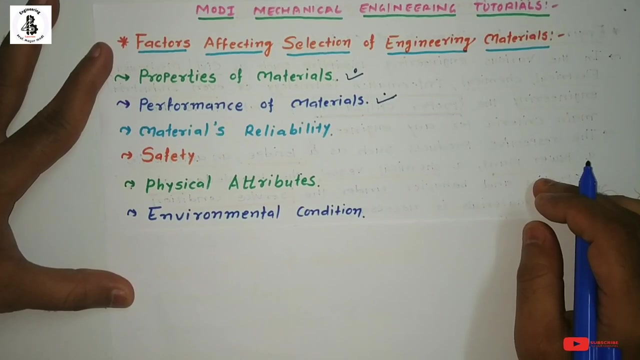 important part as a physical attributes. so that will be also considering as a factors which will be affecting the engineering materials, environmental conditions. so the working environment under which a part, or you can say, the product has to perform its function influences the service performance of it. so the basics, the 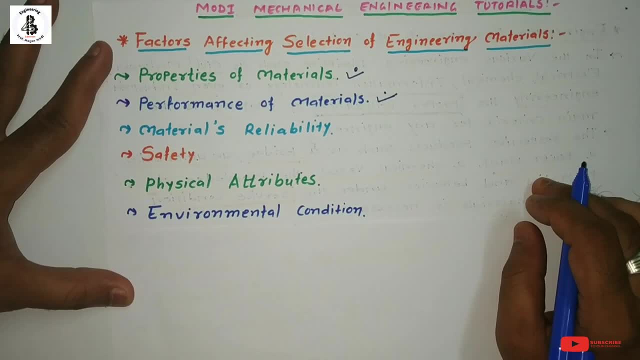 performance of temperature, humidity, water or you can say harsh chemicals in the working environment of the products can be causes the corrosions or you can say creeping of the material, so that will be reducing the life of the product. so environment that will be having a vital role for 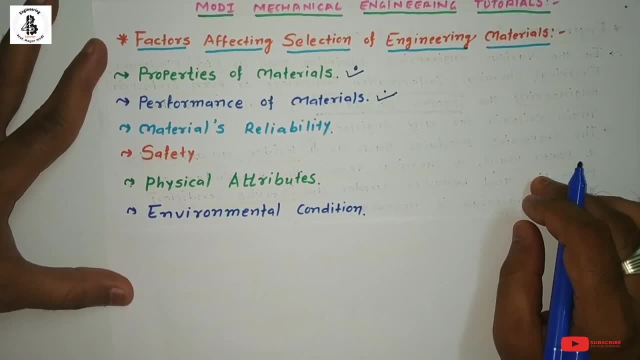 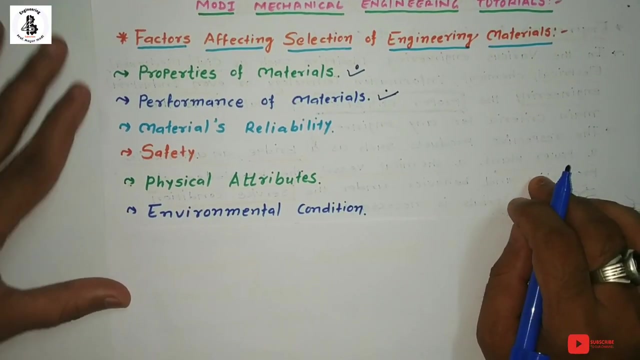 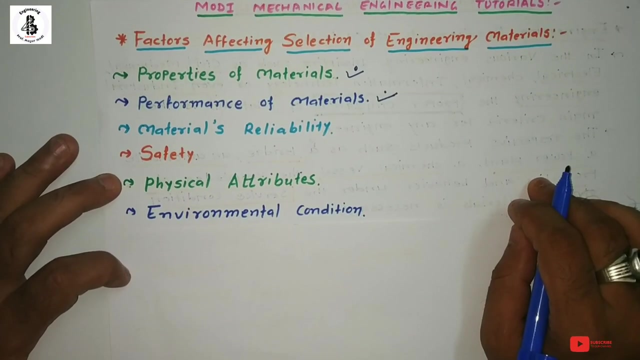 deteriorating the properties of the materials. so this will be tend to failure of the materials. so if our product it will be into the hazardous chemicals or you can say hazardous environment. so you need to select such kind of materials according to the requirements of the property, environment conditions. that will be one kind of factors which will be influencing on to the selection of the engineering materials. 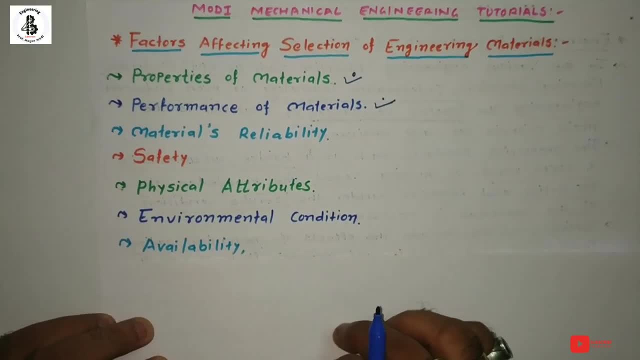 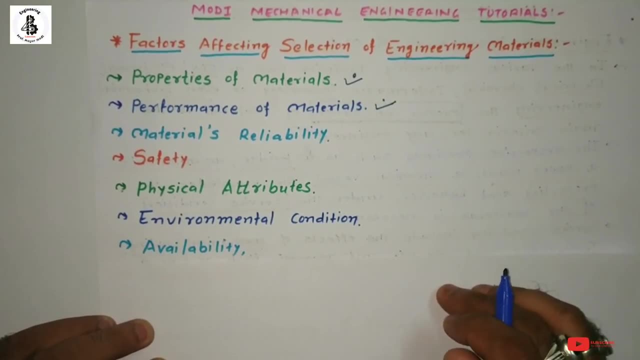 availability. so a material must be readily available and in quantity large enough for the requirement of the product, so of course that will be considering as a good quality materials. so one must be think in advance for the alternative choice of the materials when the existing material becomes available, with the difficulties So you need to controlling the. 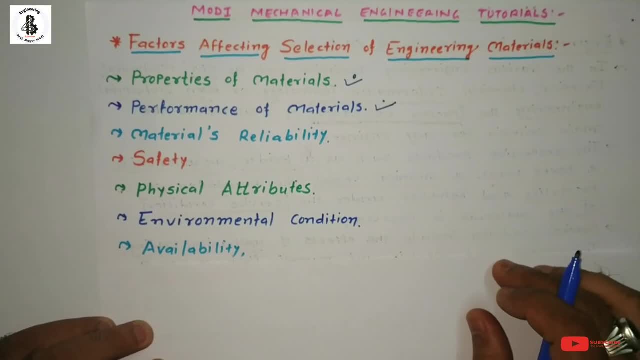 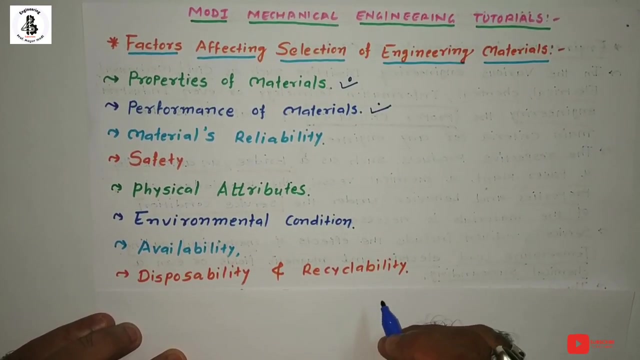 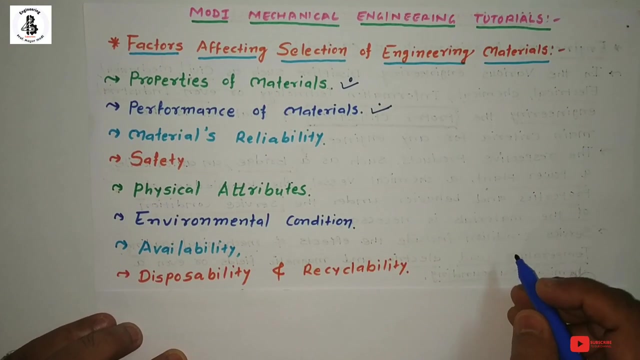 second kind of materials that will be replacing your basic materials. So availability: it will be having a vital role for getting as a raw materials Disposability and recyclability. So the selected materials should not be harm environment in the surroundings. Also, they should not produce any pollutions in any kind of form. So nowadays, government, it will be take. 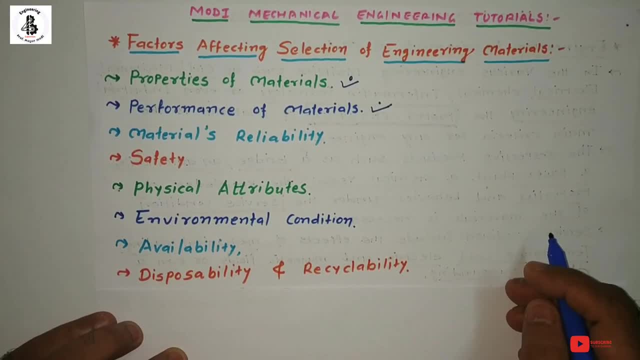 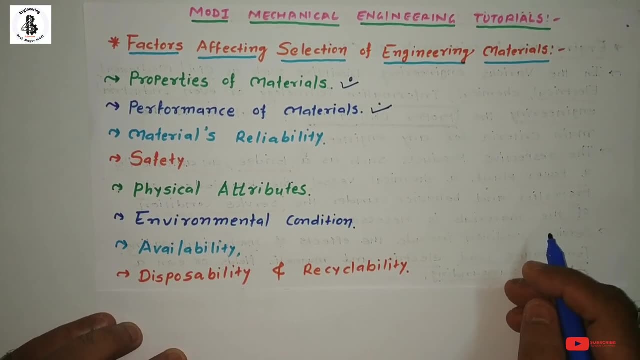 the precautions for recycling or you can say disposability of the any kind of metallic material, plastic material, you can say the waste materials. So before that will be living into the environment, you should process for the recycling or reuse of the particular products. Economic factor: 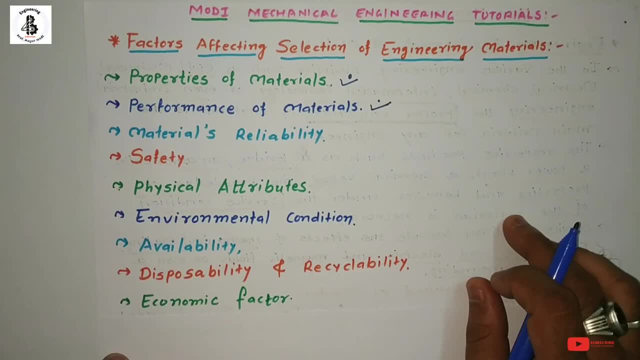 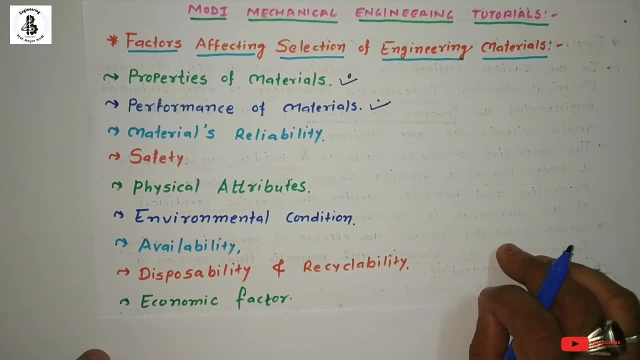 So the total cost of the any products- or you can say part or process- is the sum of the cost of the materials and the cost of the processing it into the finished product or a part. So the most important factors for the selection of materials is always the cost, because it affects 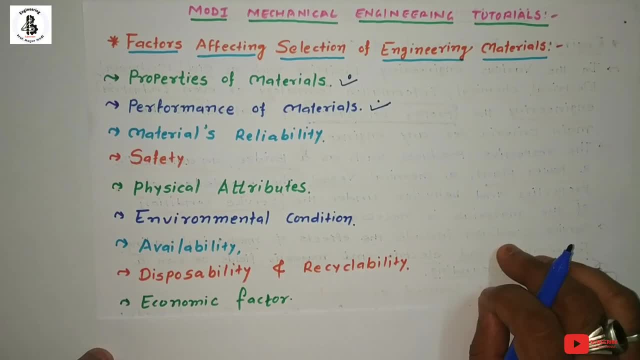 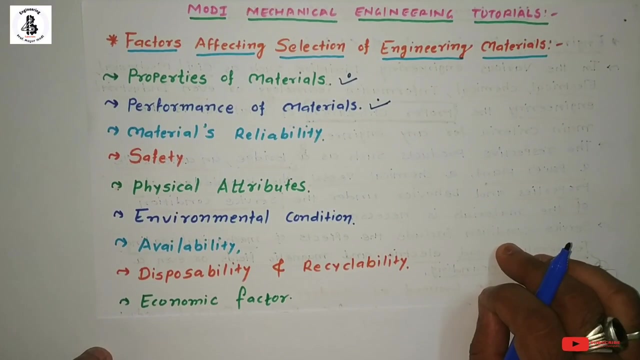 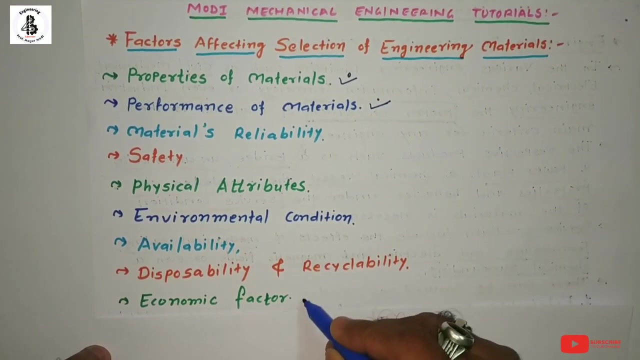 the economy of the form, or you can say industry producing the products. So there is always a limit up to the which You can afford the price. So in the form itself, The steps for reducing the cost of the product must be given due to the consideration. So all the industries that will be always focusing on, to the last price, it will be having a good properties, or you can say good, reliable materials. So that will be the most important parameter: economic factor, or you can say economic consideration. 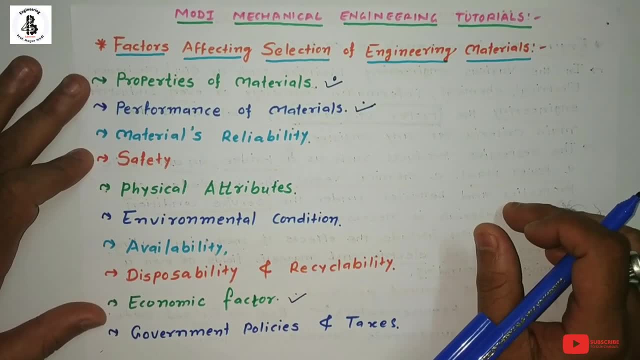 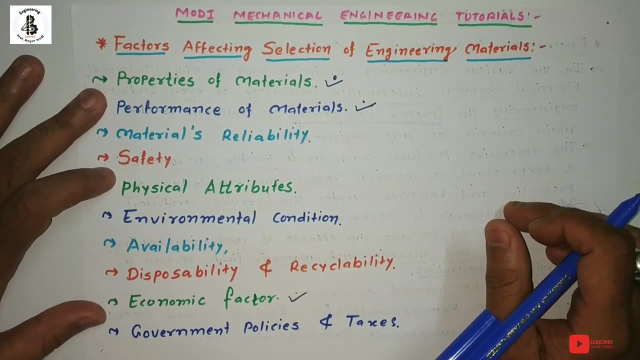 Last topic for factor affect. So one of the factors- it is actually one of the 우's most important factor- is selecting the selection of the engineering materials and that will be government policies and taxes. so many times the government policy, such as rules for the import, export, used. 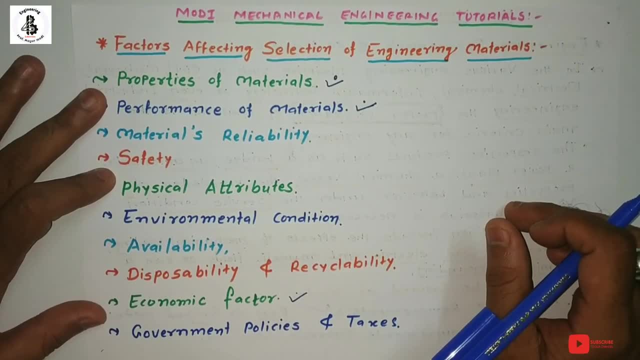 Sales tax, Excise duty- where you added tension Can say that, etc. Changes during the course of the time. so, while selecting of material, these factor Become very important. as each Decided, the companies: grill, Choose the purchase, Execute any big task you have to perform process.